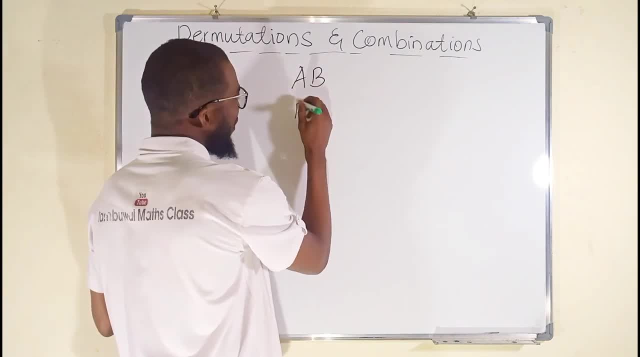 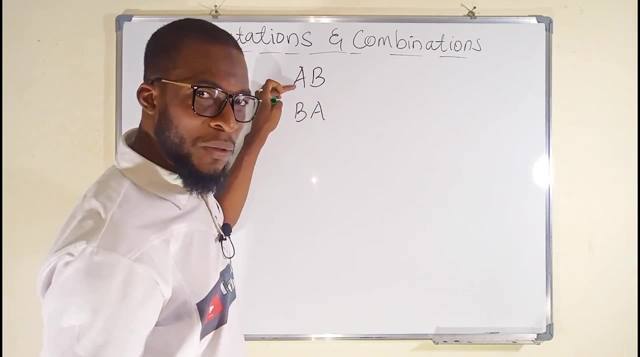 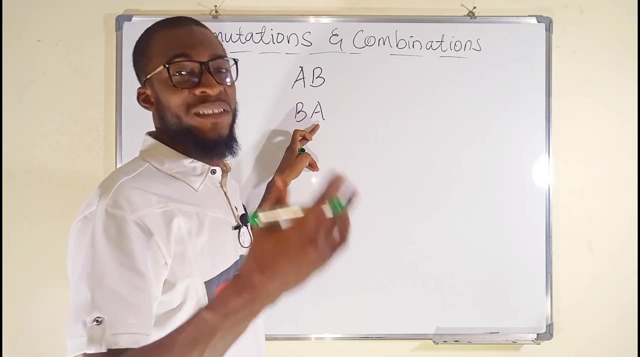 different ways: ABO, let me say BA. Can you see that we have two different arrangements? We can say ABA and ABA. Can you see that we have two different arrangements but a single combination, because AB and BA are all letters, AB, so in combination. 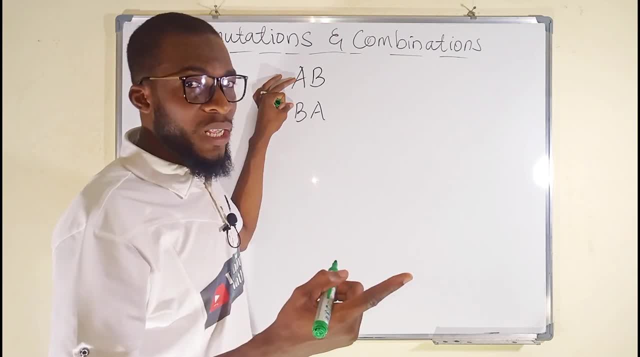 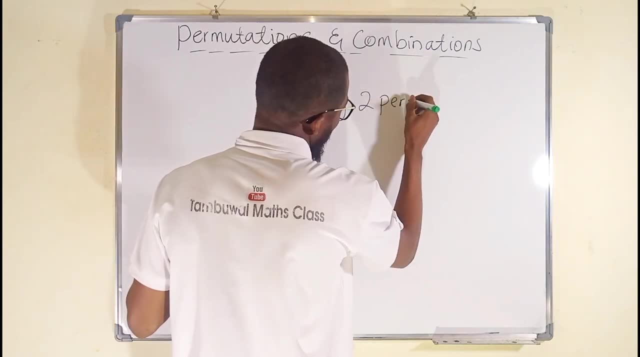 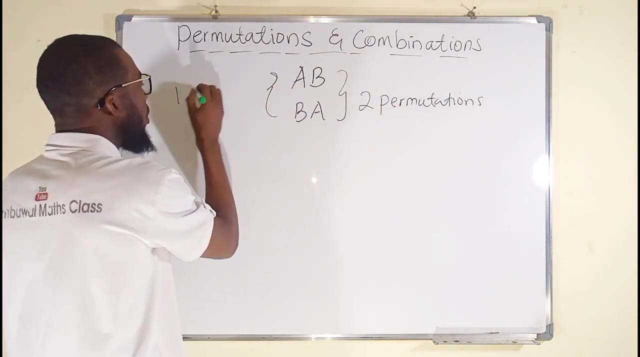 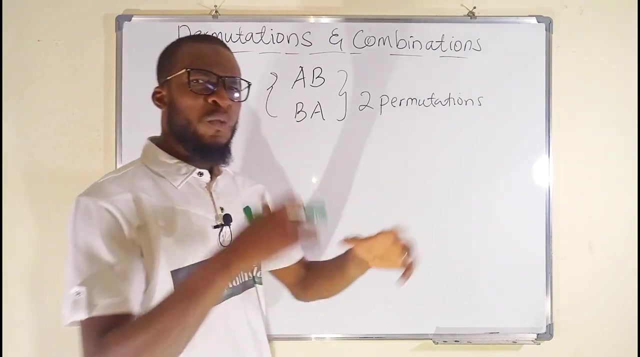 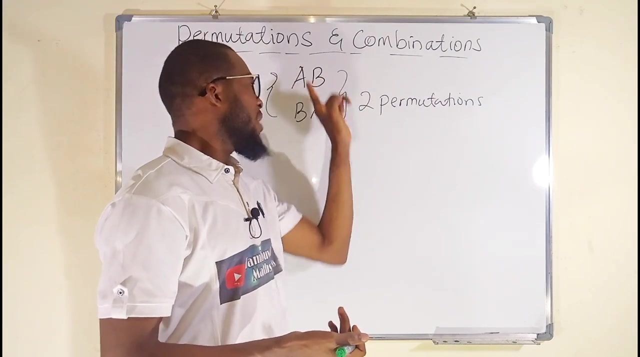 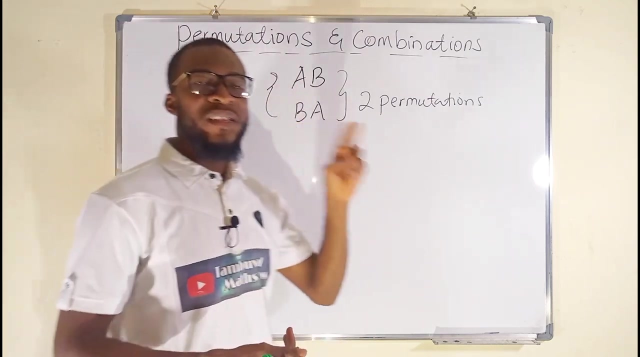 they are regarded as one, but in permutation they are considered as two. so we have two permutations here, but one combination. can you see the difference between the two? permutation is concerned with the arrangement where order does matter. AB and BA are two different arrangements in permutation, But since AB and BA are all letters AB, they are going to be considered as one combination. 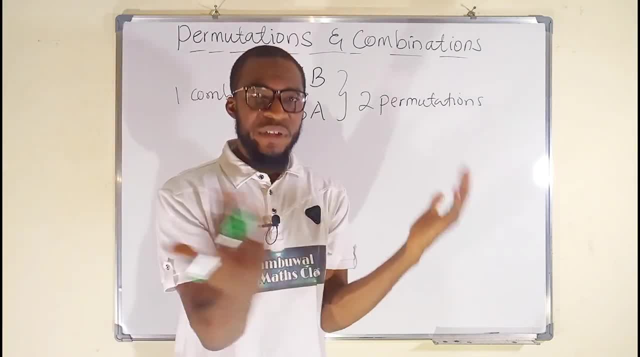 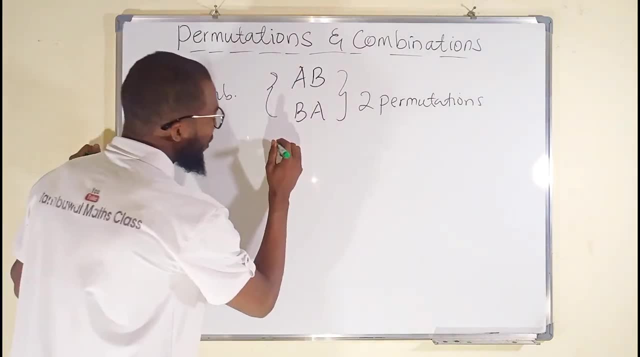 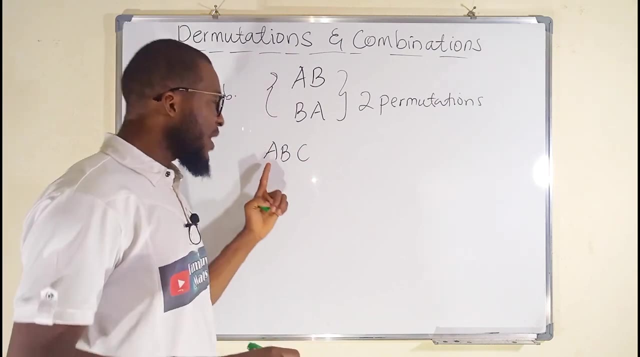 In combination order doesn't matter. No matter how you arrange it. despite they are the same letters, they are going to be considered as one. Suppose we have another one, ABC. How many ways can we arrange ABC? We can arrange it as ABC. 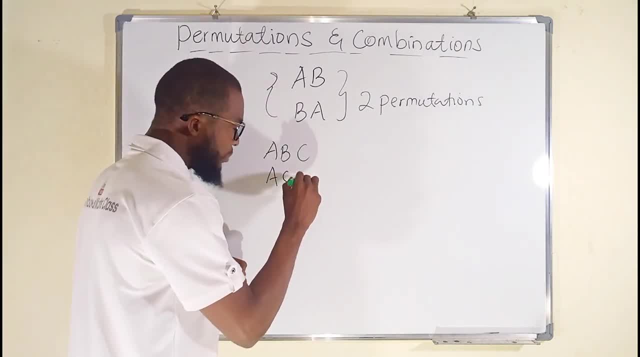 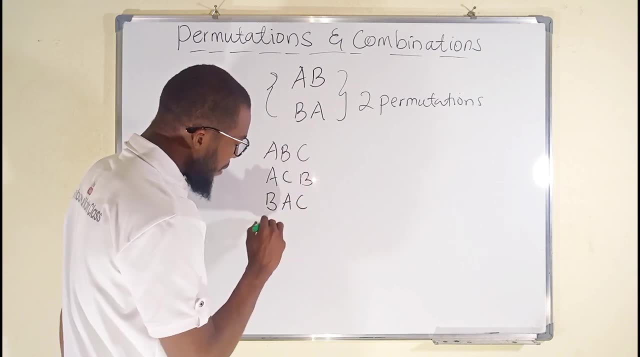 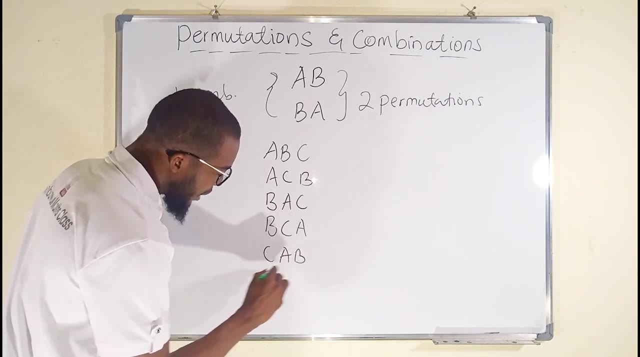 We can also arrange it as ACB. We can equally arrange it as BAC, BCA, We can arrange it as CAB and finally CBA. How many ways? 1,, 2,, 3,, 4,, 5,, 6.. 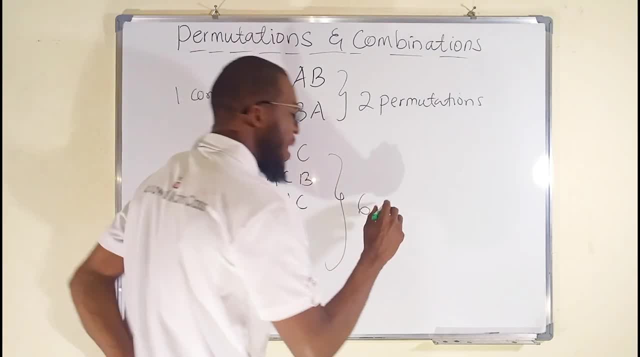 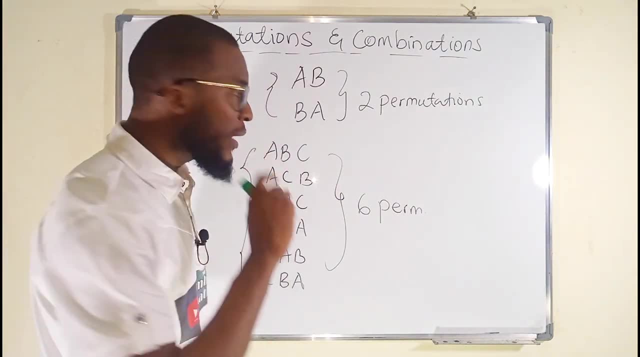 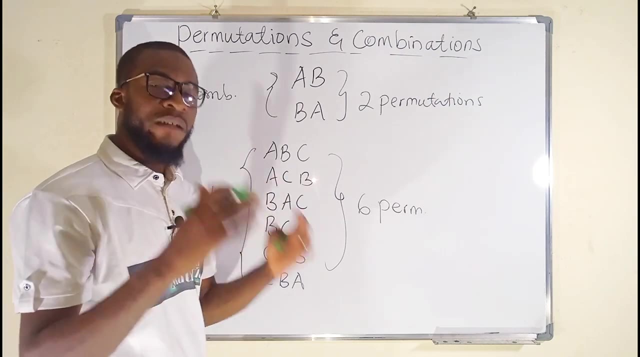 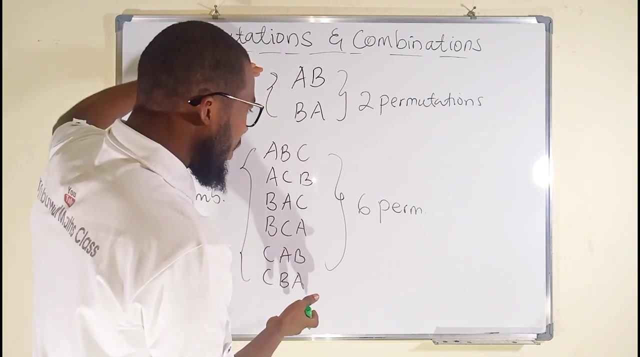 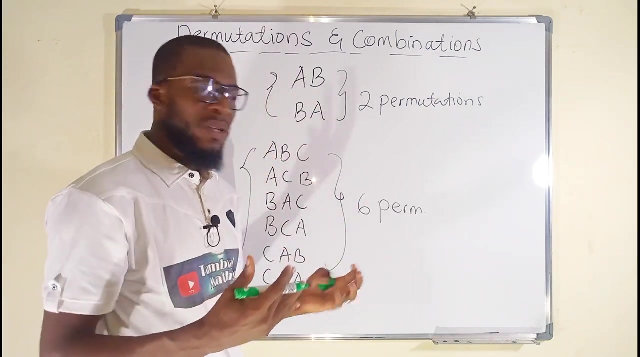 We have six different permutations, But all of these are considered as one in combination, Because they are all letters, ABC, just that they are arranged in different ways. So the arrangement of these letters in different forms is what permutation is telling us, But irrespective of the order in which they are arranged, it's what the combination is talking about. 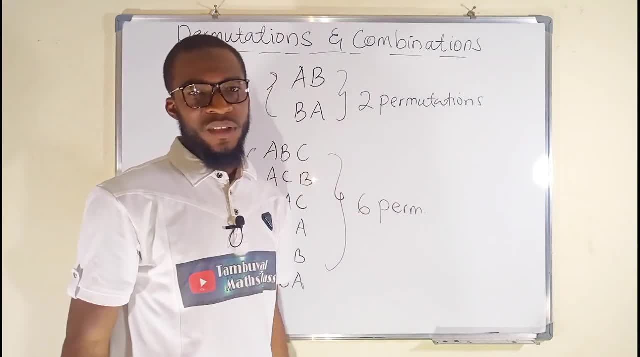 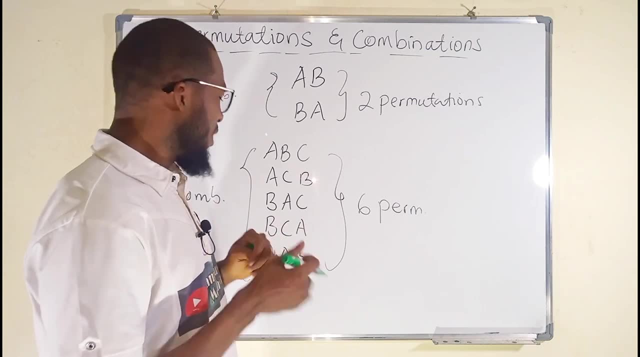 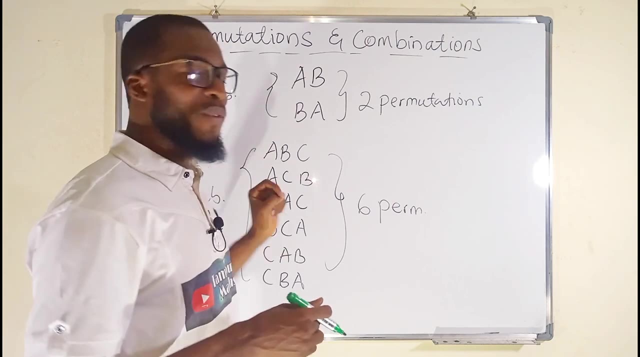 So we have one, One combination, six permutations. So this is where the term factorial comes to play. Observe something here. Let me start with this one. We have three items, but we have arranged them in six different places or in six different ways. 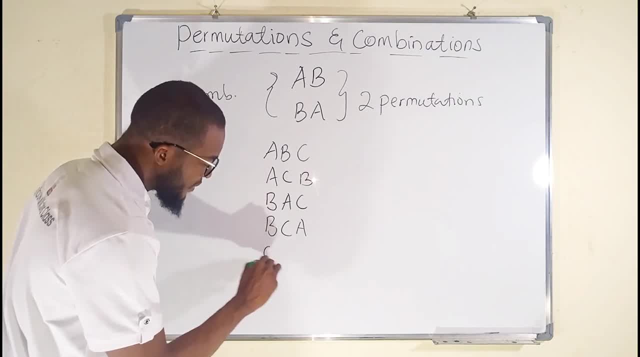 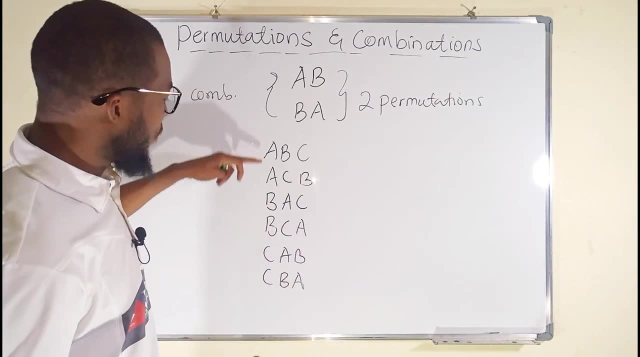 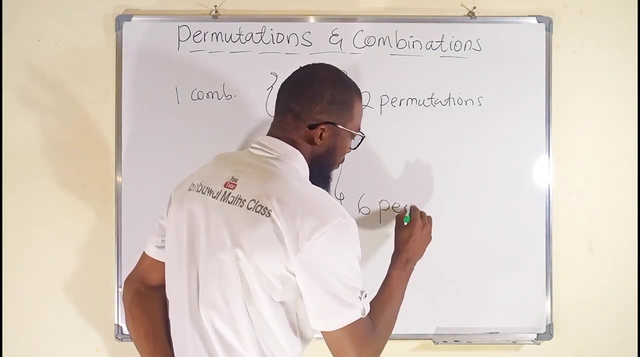 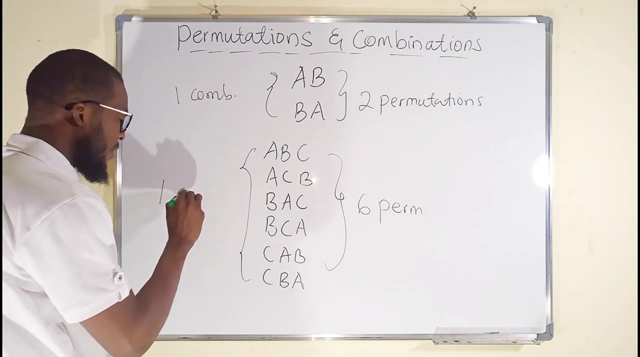 a, C, A, B and finally C, B, A. How many ways? One, two, three, four, five, six. We have six different permutations, But all of these are considered as one in combination because they are all letters: A, B, C. 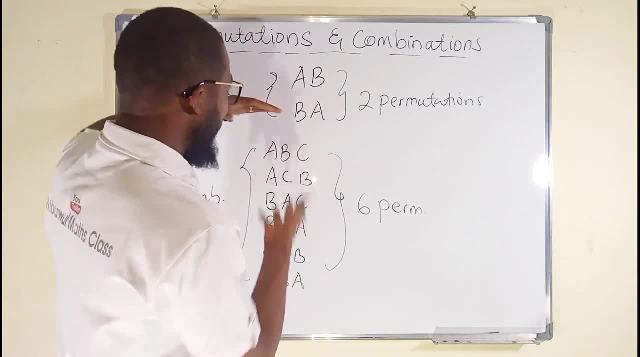 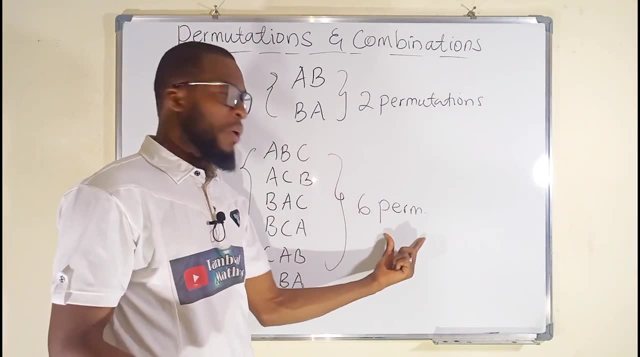 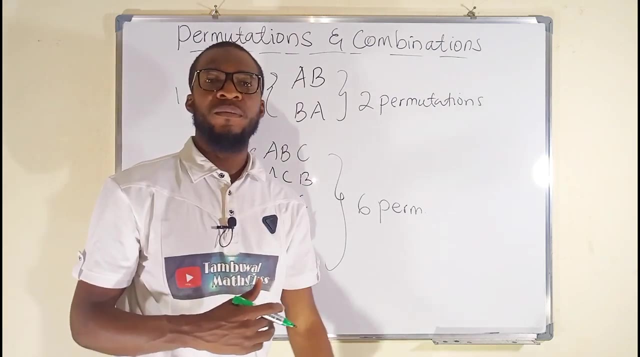 just that they are arranged in different ways. So the arrangement of these letters in different forms is what permutation is telling us, But irrespective of the order in which they are arranged is what the combination is talking about. So we have one combination, six permutations. 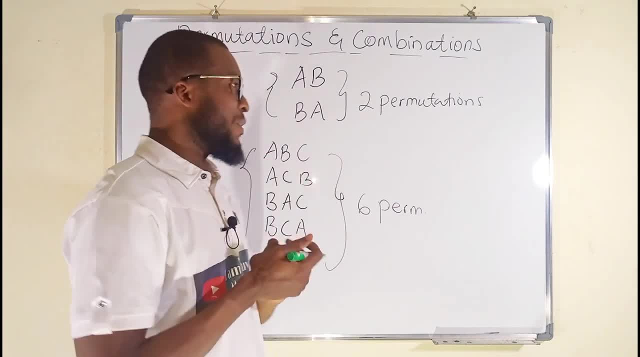 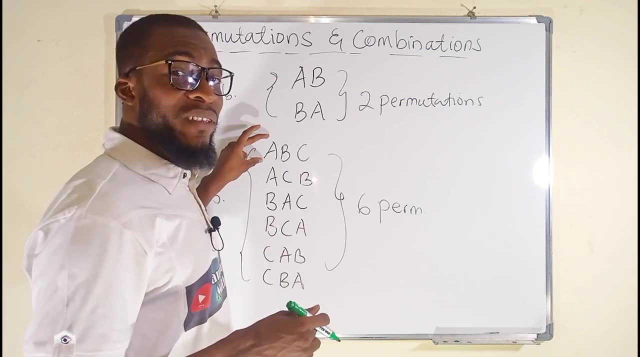 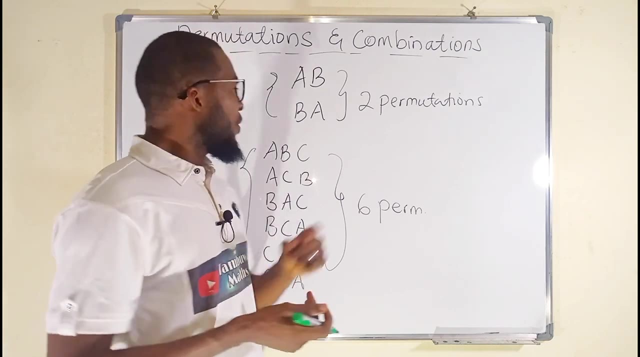 So this is where the term factorial comes to play. Observe something here. Let me start with this one. We have three items, but we have arranged them in six different places or in six different ways. To choose which number comes first, you have three options. 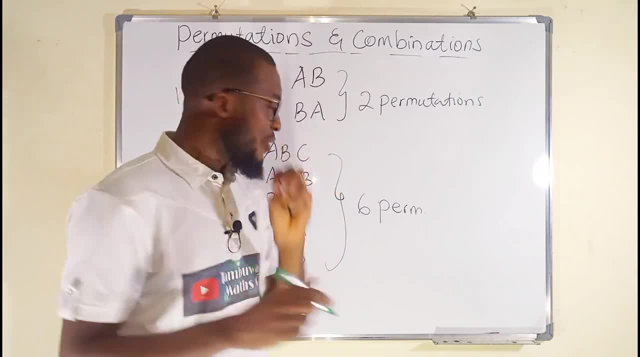 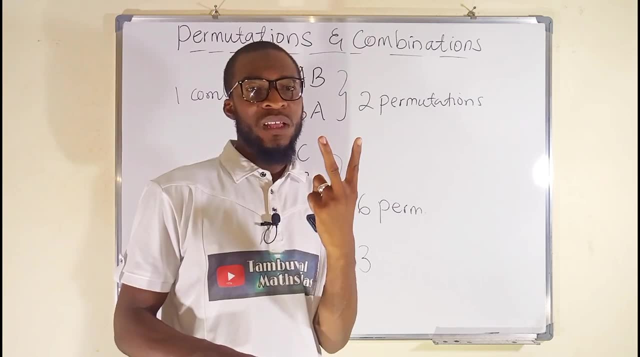 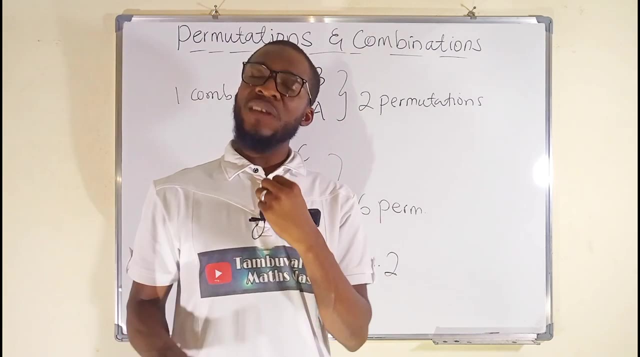 The first letter could ever be A, B or C- Three options- But having chosen the first option, you have two letters left And you have to choose among the two letters to decide which one comes second After choosing the second one. 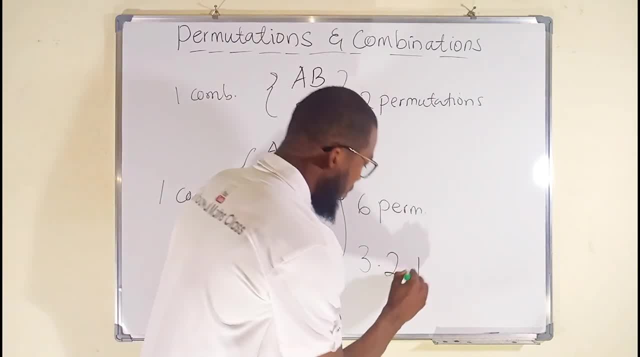 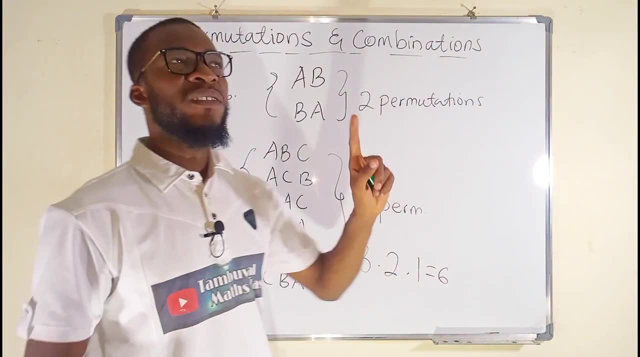 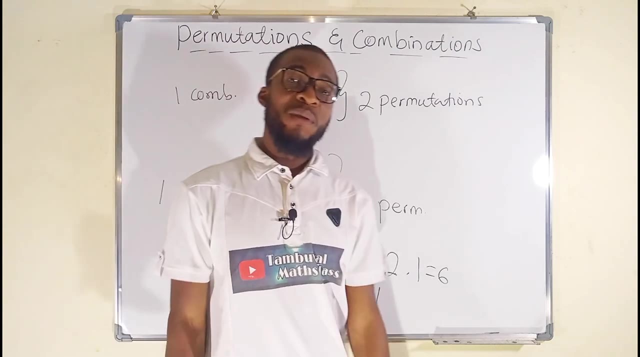 you have only one letter left, which is one. Can you see that Two times three times two times one is equal to six, And this is just a definition of factorial. This is equal to three factorial, Remember. factorial means that number or a letter. 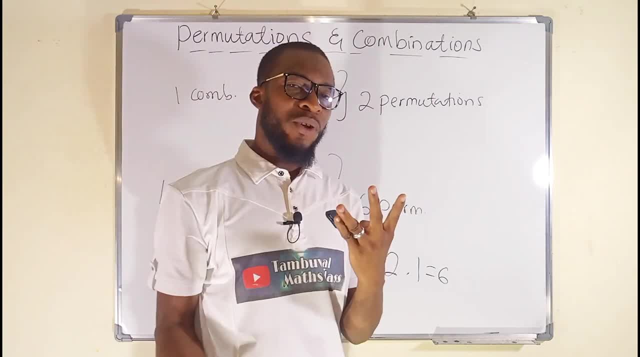 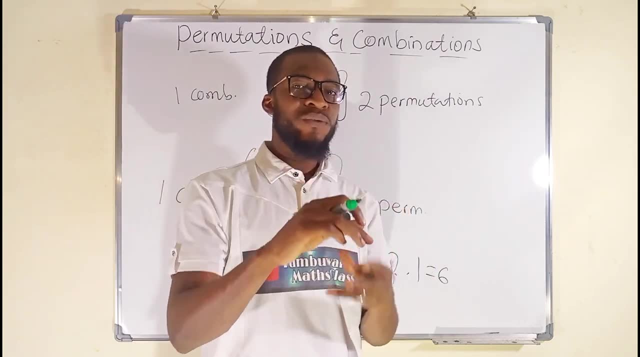 multiplied by the next number before it, multiplied by the next number before it, multiplied by the next number before it. If you have five factorial, it means five times four times three times two times one. If it is six, six down to one, 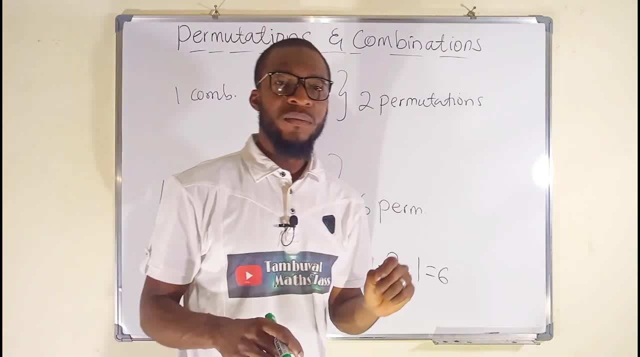 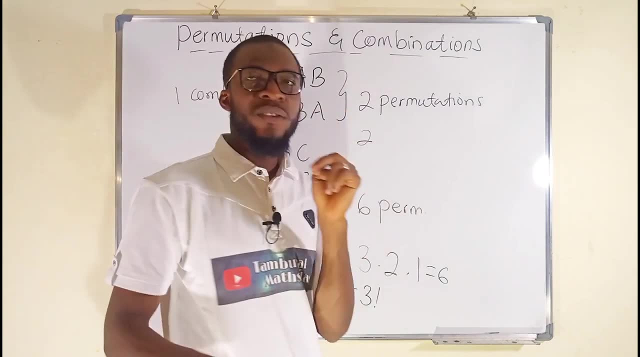 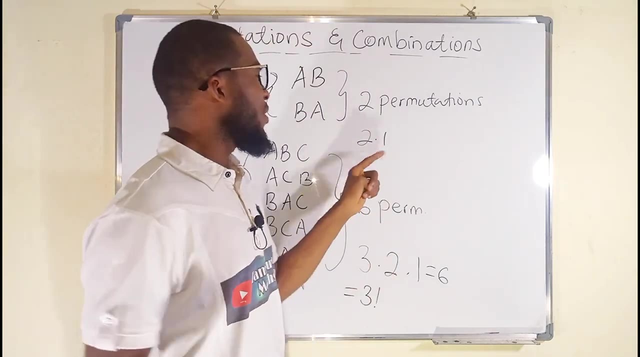 Coming here. we have two letters To choose. which letter comes first. you have to choose among the two, So we have two. Having chosen the first letter, you have one left. So that is which is going to be considered next. 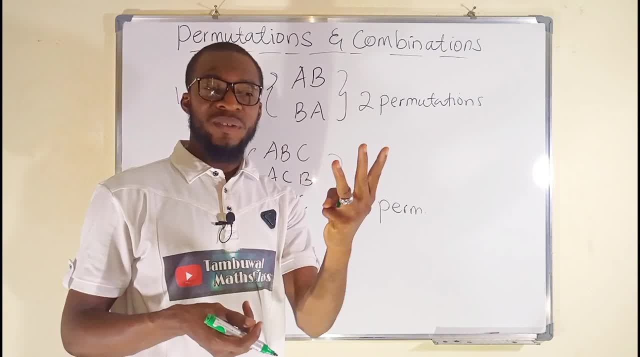 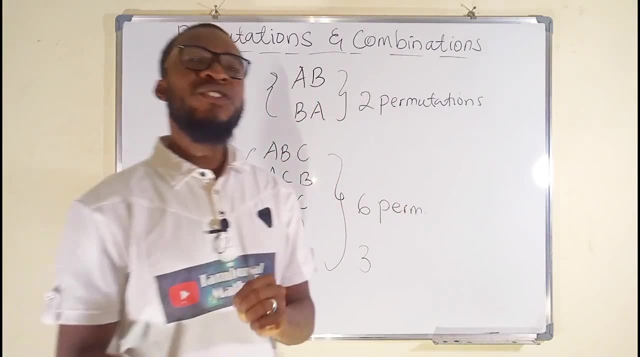 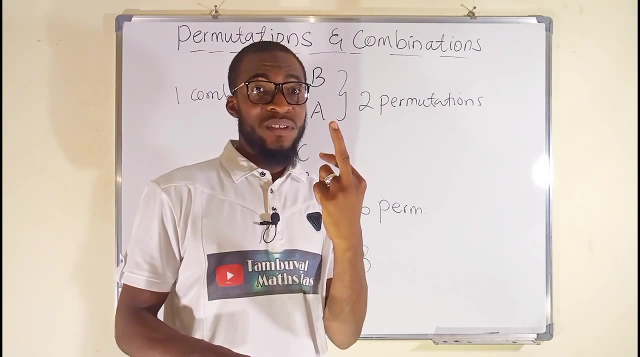 To choose which number comes first. you have three options. The first letter could ever be A, B or C- Three options- But having chosen the first option, you have two letters left And you have to choose among the two letters to decide which one comes second. 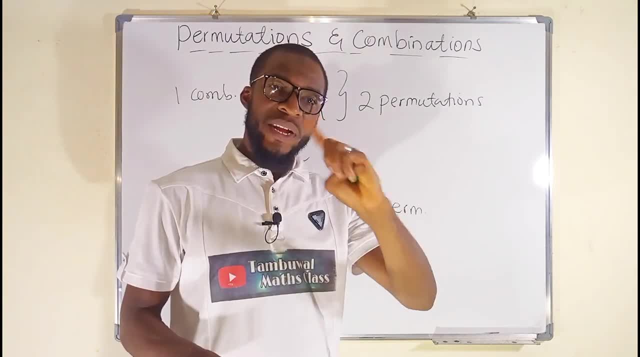 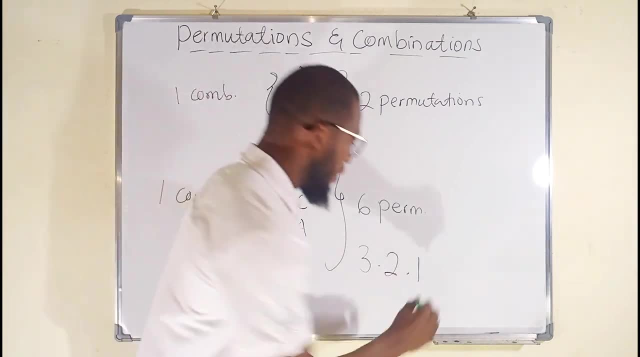 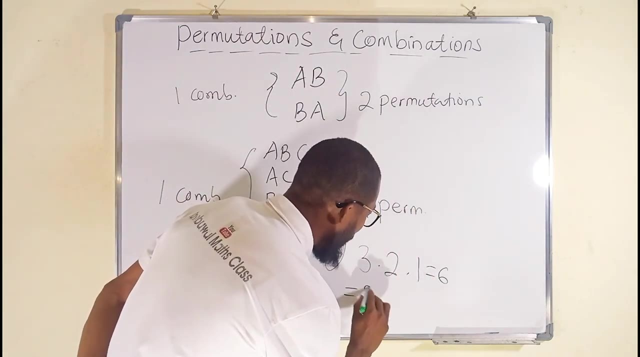 After choosing the second one, you have only one letter left, which is one. Can you see that Two times three times two times one is equal to six, And this is just a definition of factorial. This is equal to three. 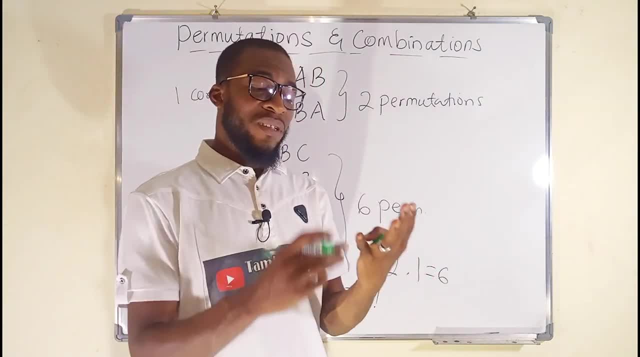 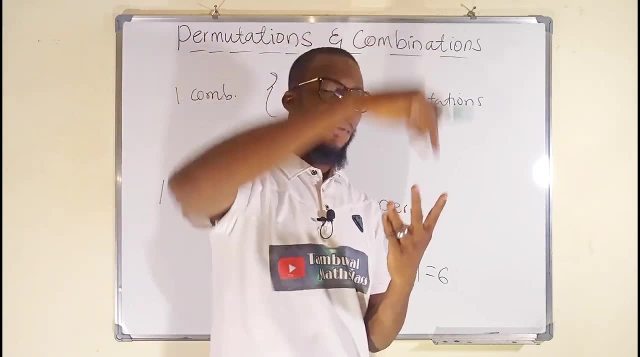 Remember, factorial means that number or a letter multiplied by the next number before it, multiplied by the next number before that one, up to one. If you have five, factorial it means five times four times three times, two times one. 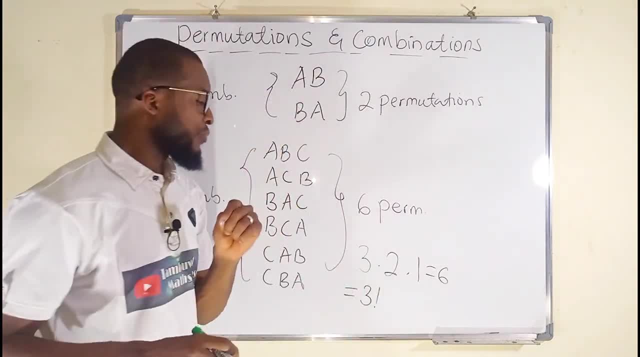 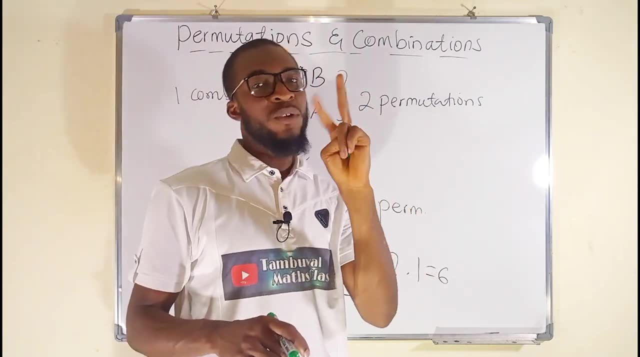 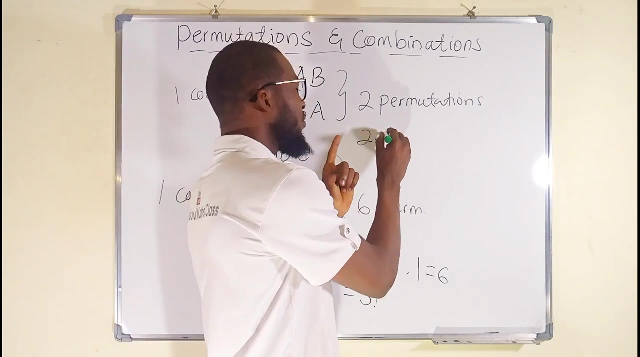 If it is six, six down to one, Come in here. We have two letters To choose. which letter comes first? you have to choose among the two. So we have two. Having chosen the first letter, you have one left. So that is which is going to be considered next. 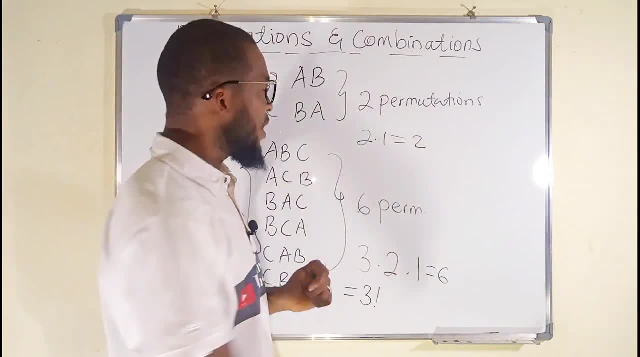 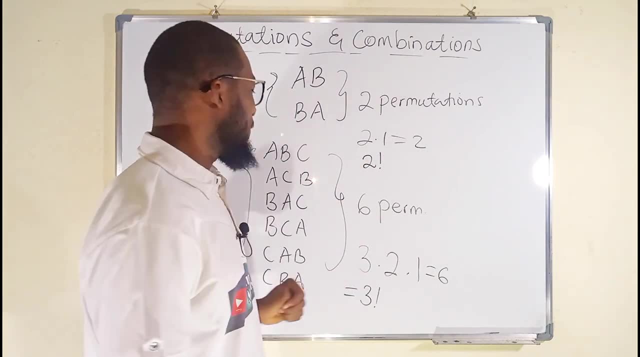 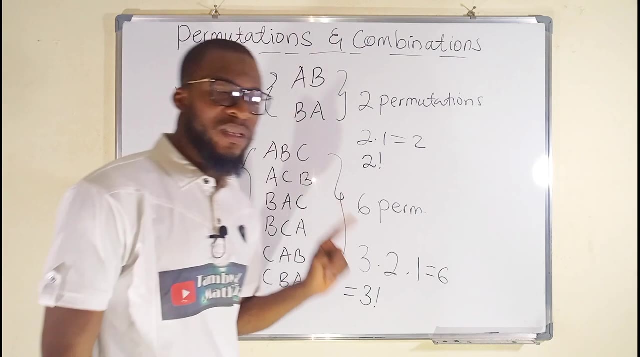 Two times one equal to two. This is why we have two permutations here, And two times one is the same thing as two factorial. All right, Coming back to combination, No matter how many times you arrange A, B, C, you will always have a single combination. 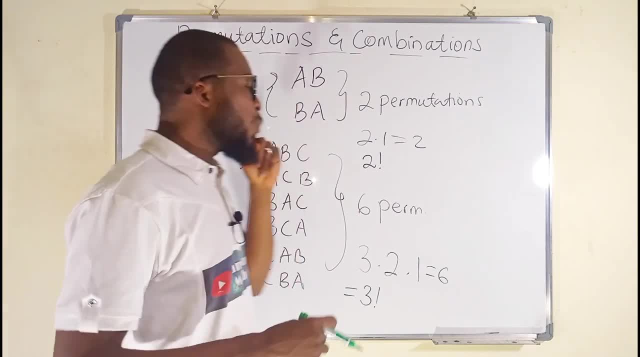 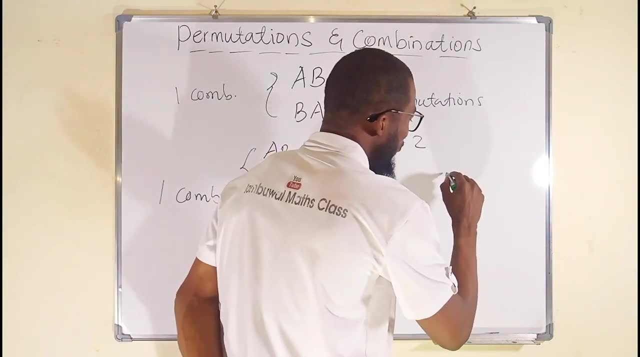 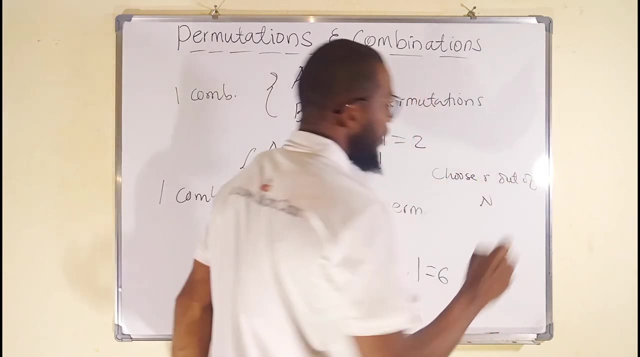 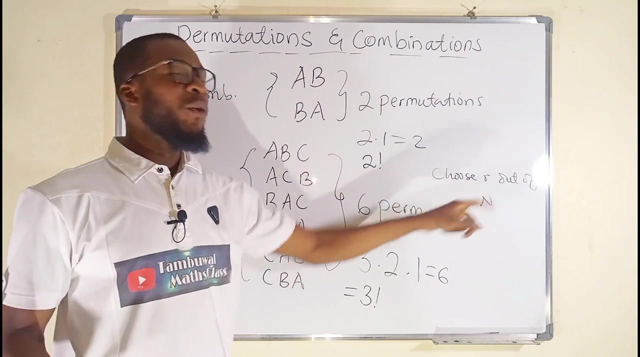 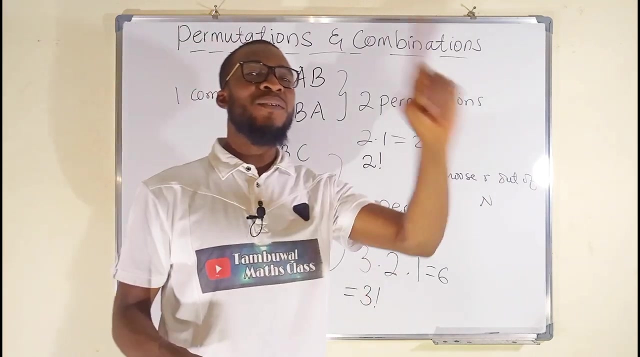 The only time you will have a different combination is when you decide to choose some r combination out of the total. maybe you want to choose r out of n, where n is the total number- like here we have abc- n is equal to 3, while r could either be 1, 2 or 3. so if r is equal to n, you will always have a. 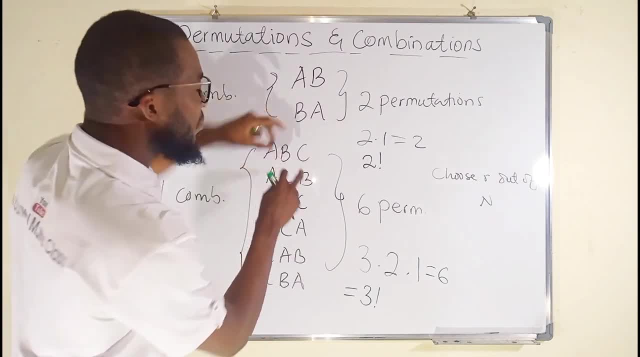 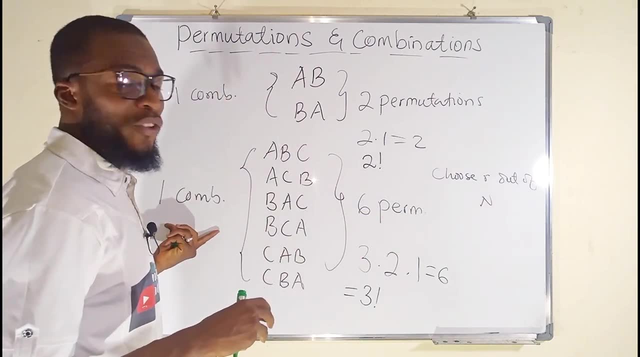 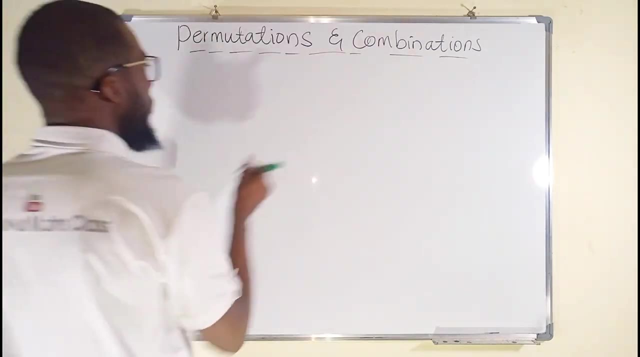 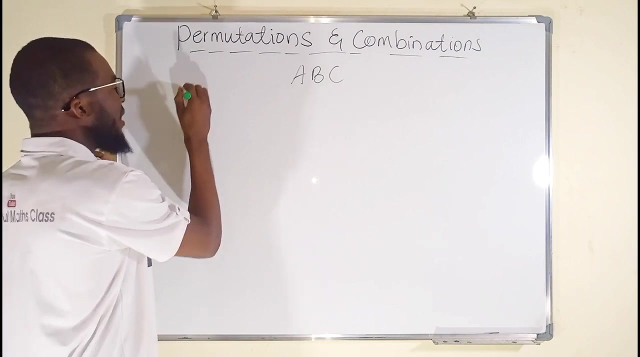 single combination, because here we have three items and we are choosing the whole three. r is equal to n. we have a single combination. but what if you decide to choose two out of three? let us do that. i'll see so first. we have a, a, a, b and c and we want to choose two at a time. we can have a b right, choosing two out of three. 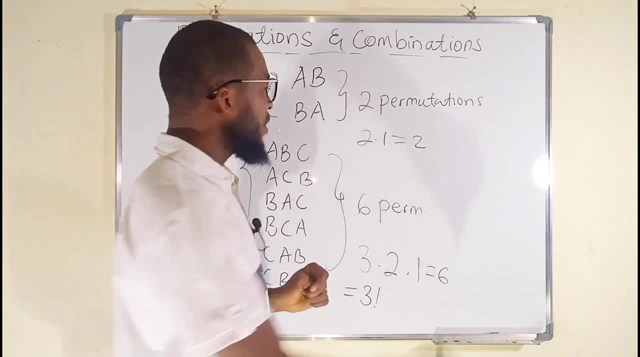 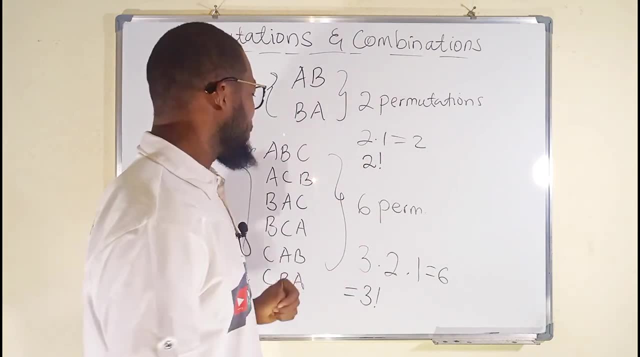 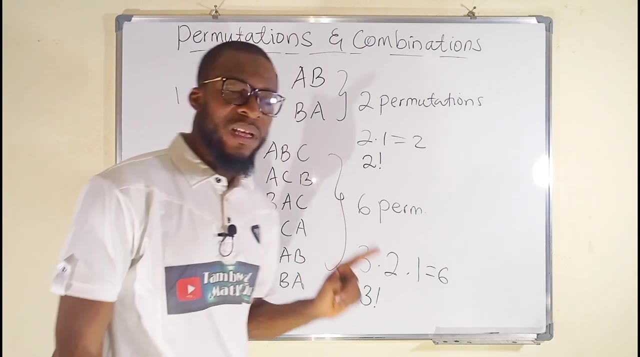 Two times one equal to two. This is why we have two permutations. We have two permutations here And two times one is the same thing as two factorial. All right. Coming back to combination, No matter how many times you arrange A, B, C. 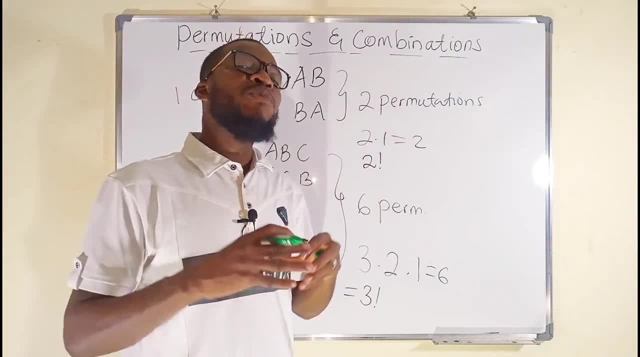 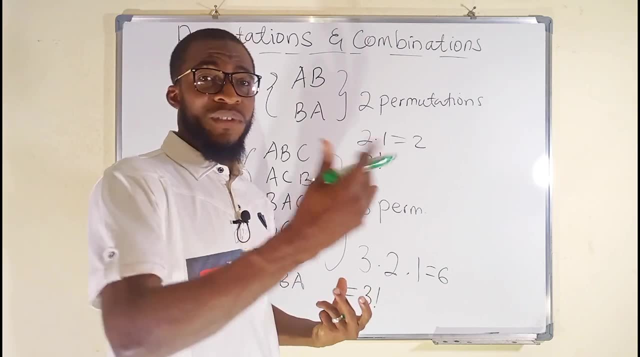 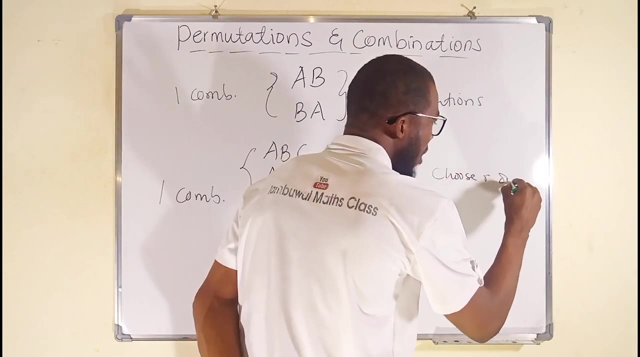 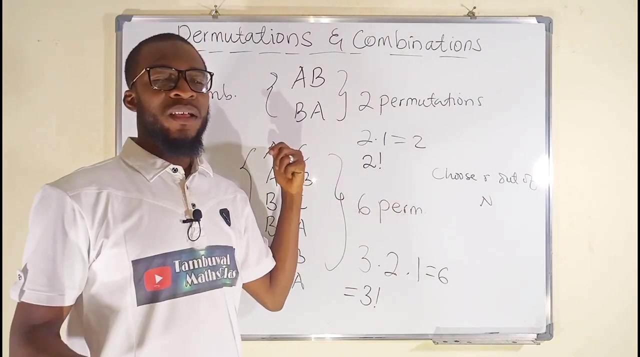 you will always have a single combination. The only time you will have a different combination is when you decide to choose some R combination out of the total. Maybe you want to choose R out of N, Where N is the total number, like here we have A, B, C, N is equal to three. 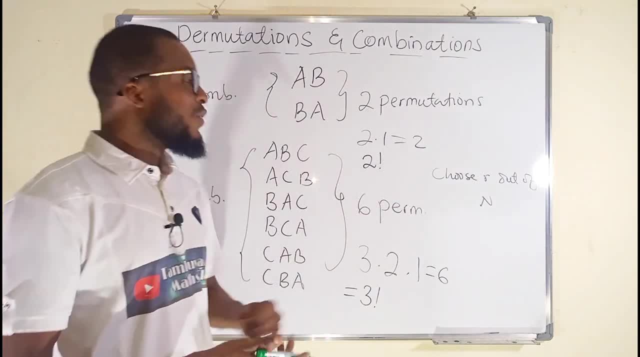 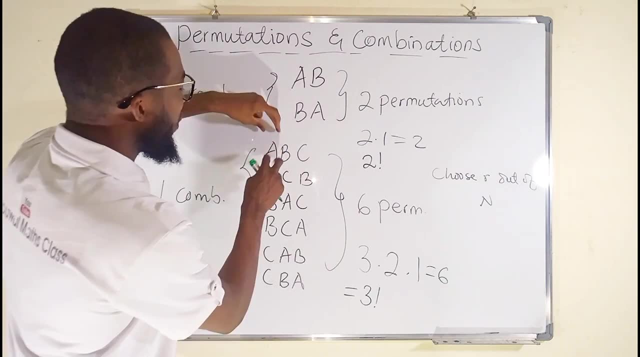 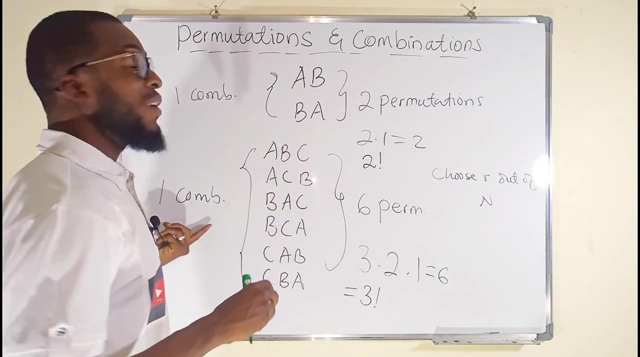 Where R could either be one, two or three. So if R is equal to N, you will always have a single combination, Because here we have three items and we are choosing the whole three. R is equal to N, We have a single combination. 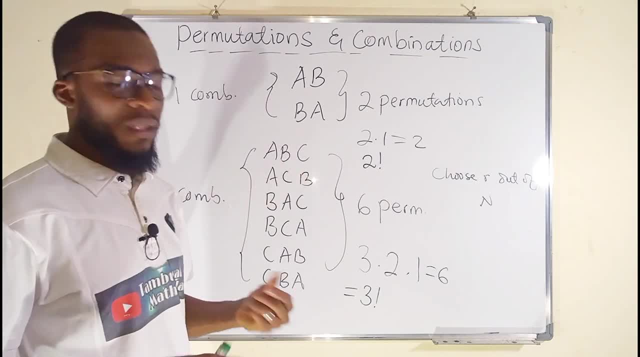 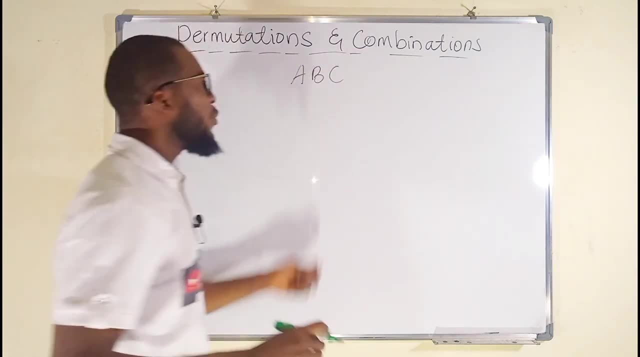 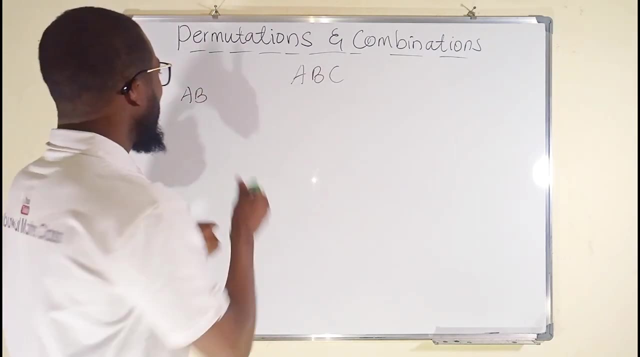 But what if you decide to choose two out of three? Let us do that and see So. first, we have A, B and C And we want to choose two at a time. We can have A- B right, Choosing two out of three. 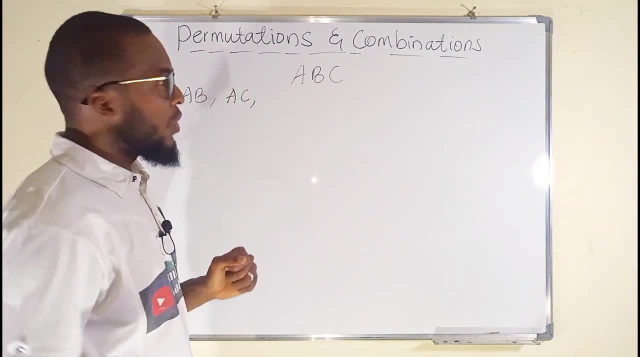 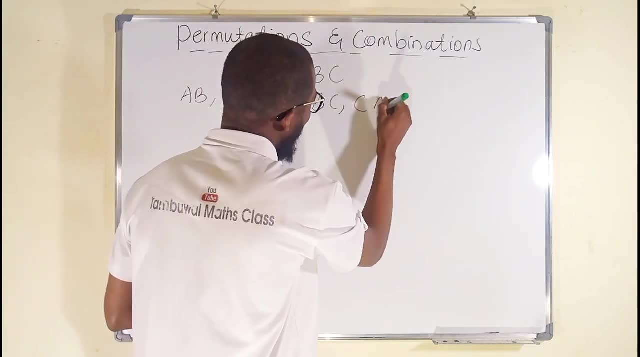 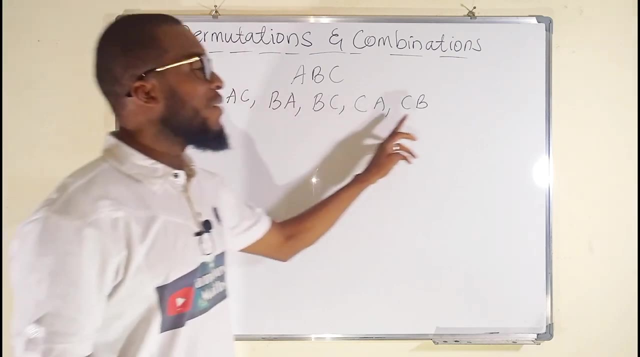 We can have A C, We can have B A, We can have B C, We can have C A And, lastly, we can have A, B C And lastly C B. One, two, three, four, five, six. 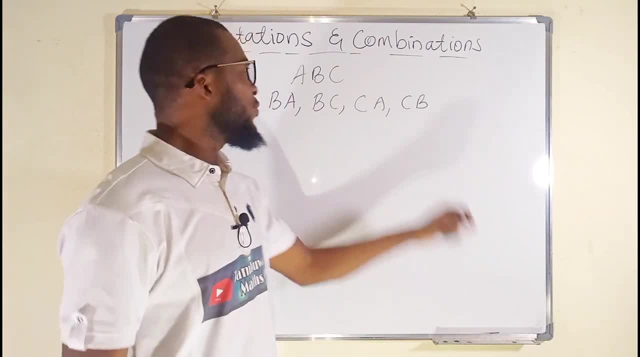 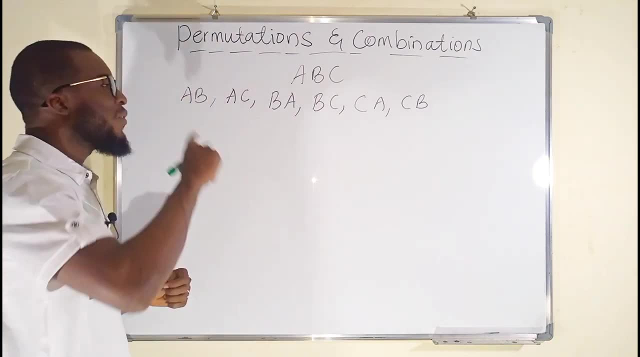 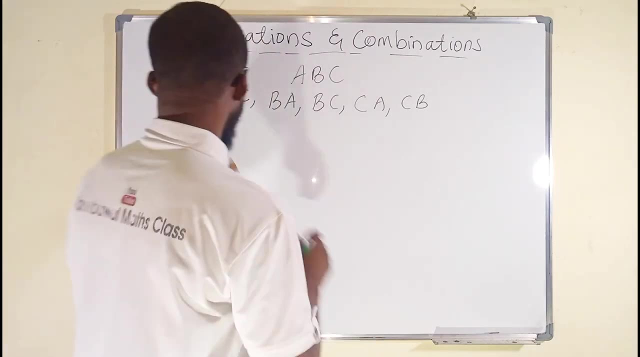 We have six different permutations in choosing two out of three. We're in arranging two out of three, But we have only three combinations here Because, remember, order doesn't matter in combination. So A, B and B- A are all the same thing in combination. 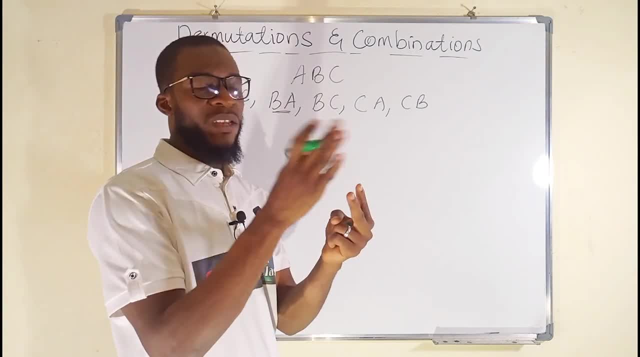 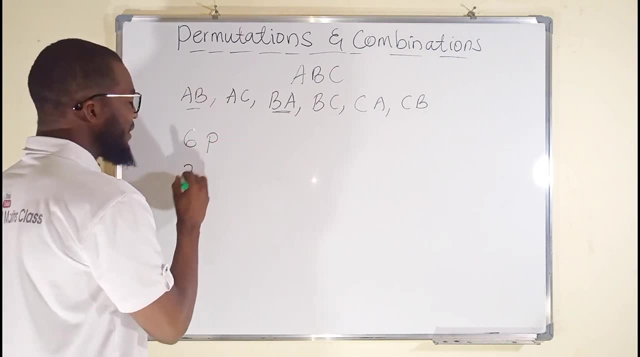 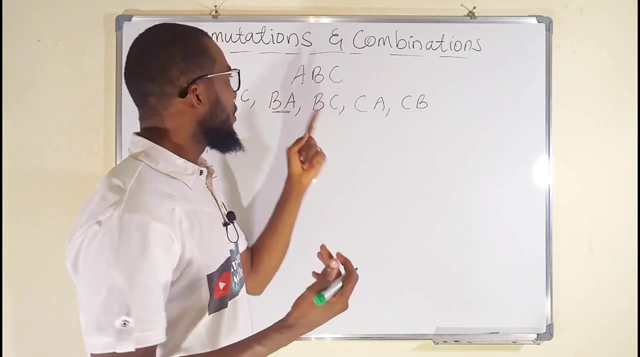 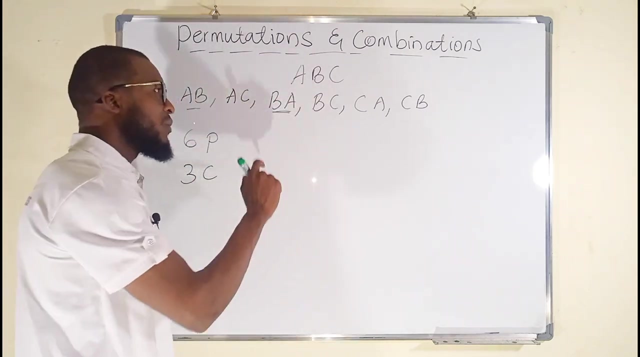 There are two numbers interchanged in different places. So we have six permutations, but what? Three combinations. This brings us to an important formula that would always guide us in deciding the number of permutations and combination in a group of items. Okay, let us apply this as an example. 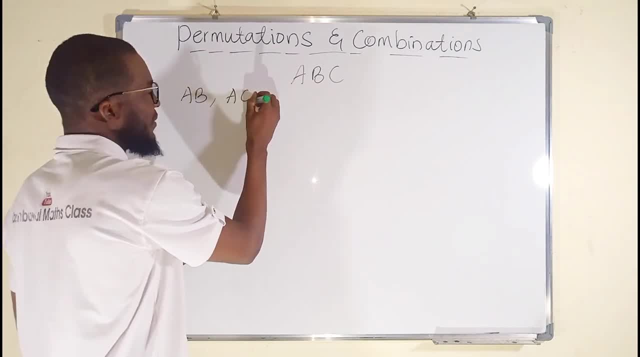 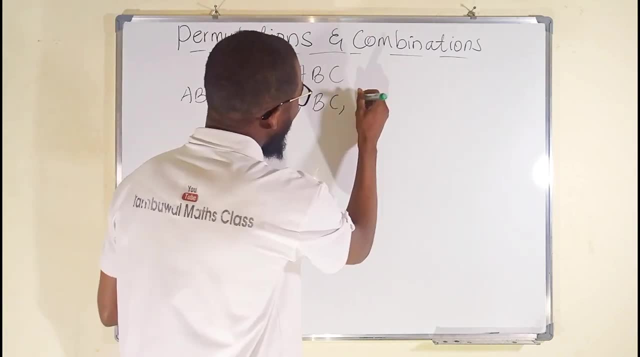 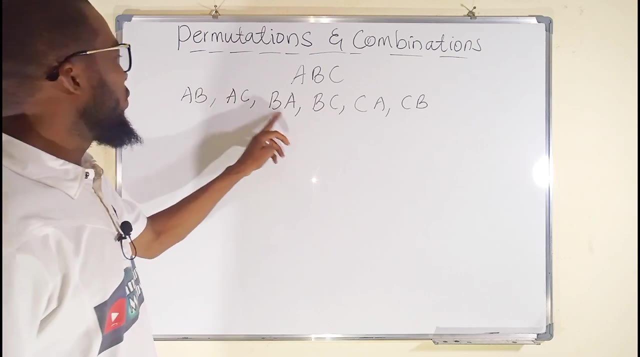 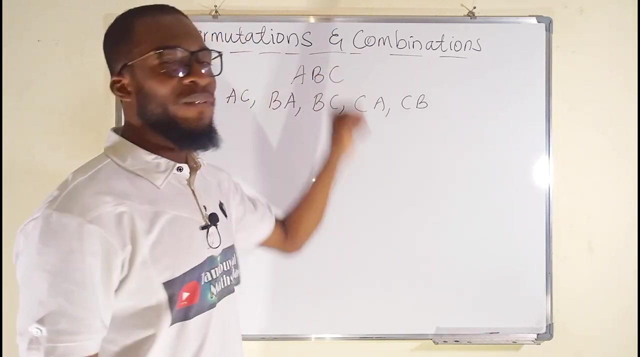 we can have a c, we can have b a, we can have b c, we can have c a and, lastly, c, b, b, 1, 2, 3, 4, 5, 6. we have six different permutations. we have six different permutations in choosing two out of three. 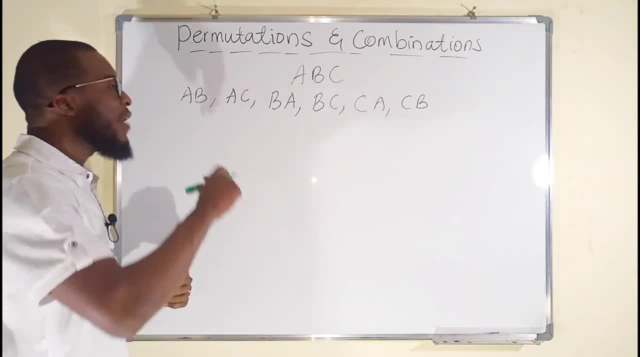 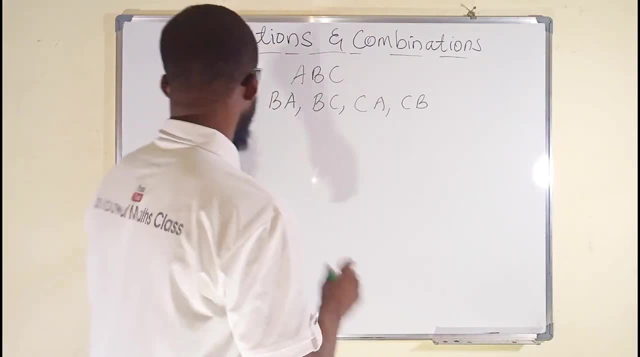 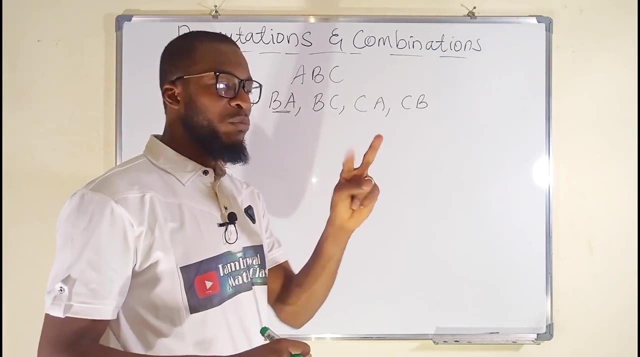 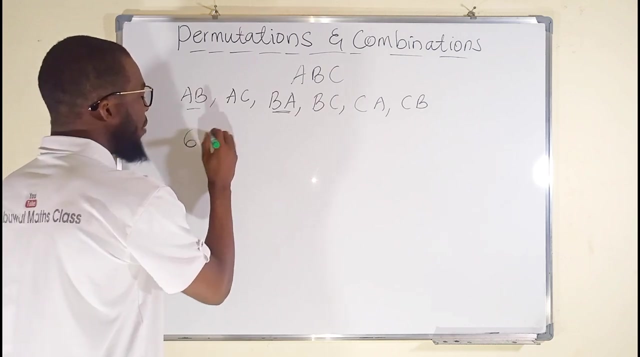 or in arranging two out of three. but we have only three combinations here because, remember, order doesn't matter in combination. so a, b and b, e are all the same thing in combination. there are two numbers interchanged, uh, in different places, so, and we have six permutations. we have 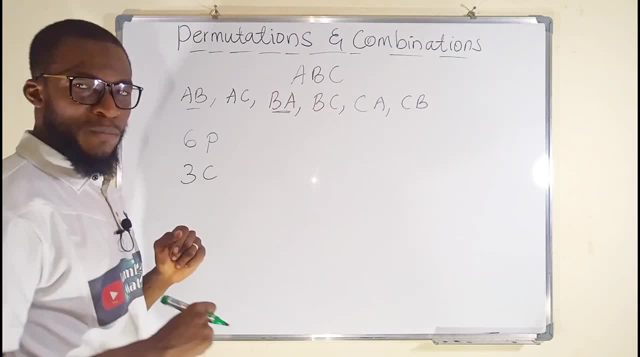 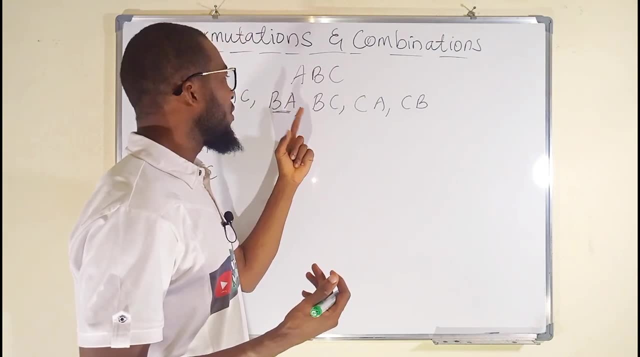 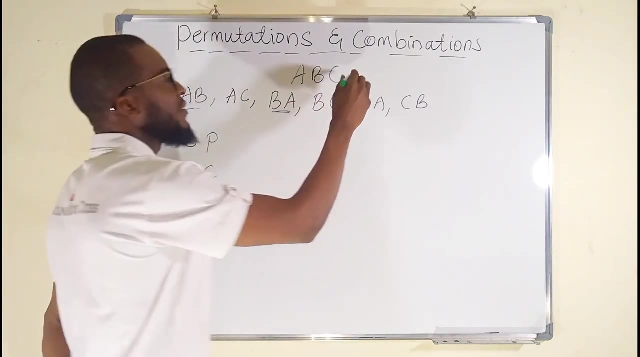 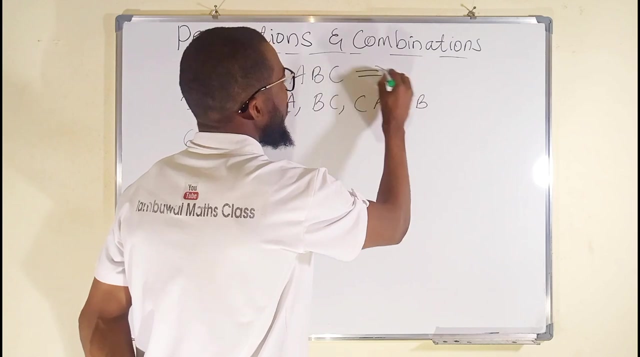 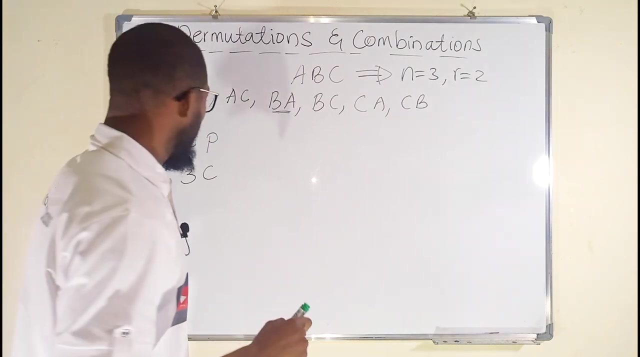 but what three combinations? this brings us to an important formula that would always guide us and deciding the number of permutations and combination in a group of items. okay, let us apply this as an example where n here is equal to 3 and are n equal to 3 and are equal to 2, because we are choosing 2 out of 3. so 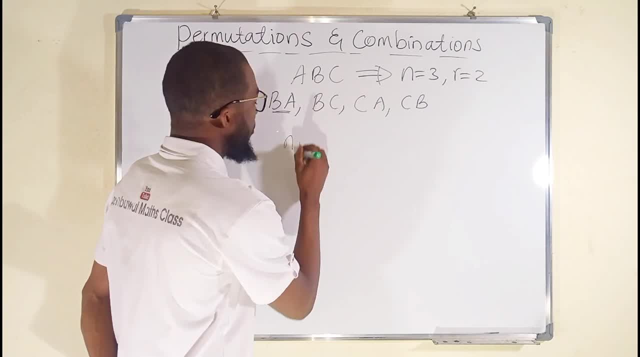 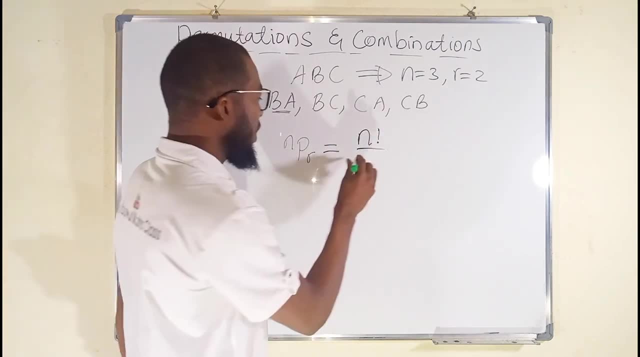 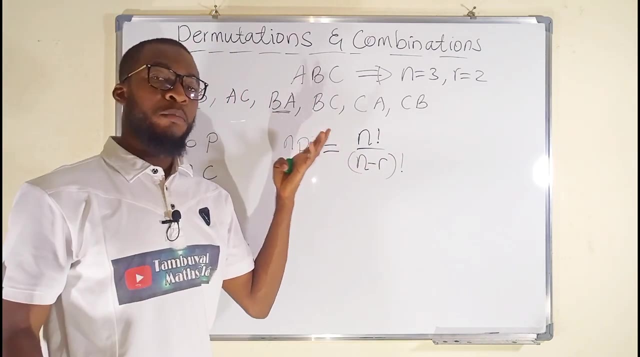 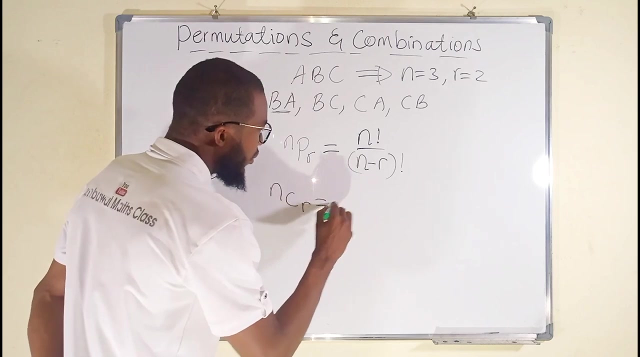 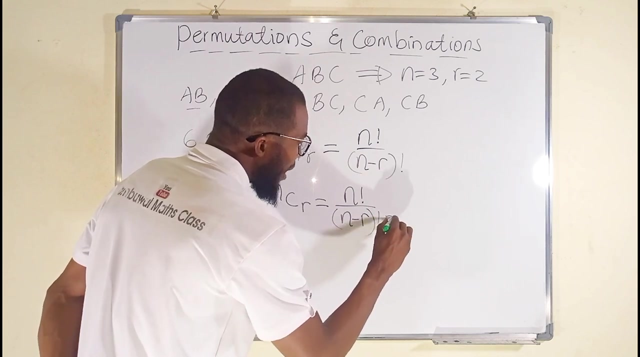 for permutation we have n permutation, r, which is equal to n factorial- remember we know what n factorial is all about- divided by n minus r factorial. this is what defines permutation. but for combination we have n choose: r is equal to n factorial divided by n minus r factorial, then also multiplied by r factorial. 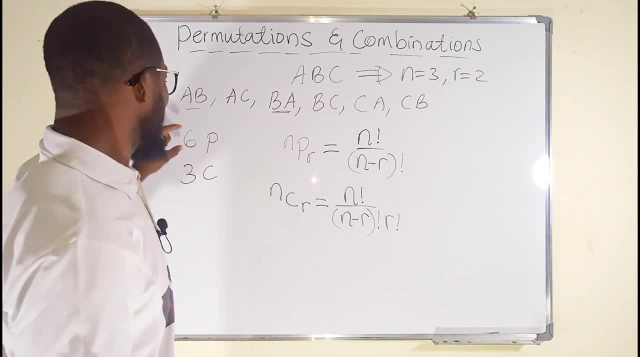 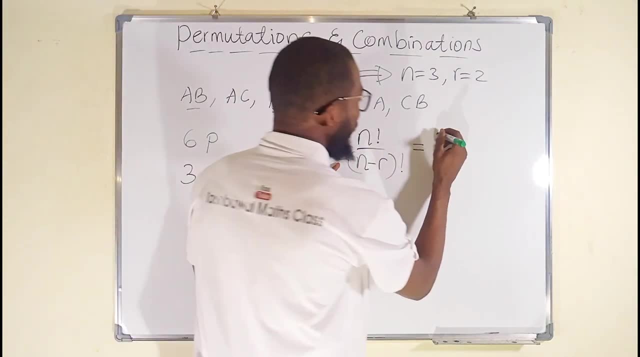 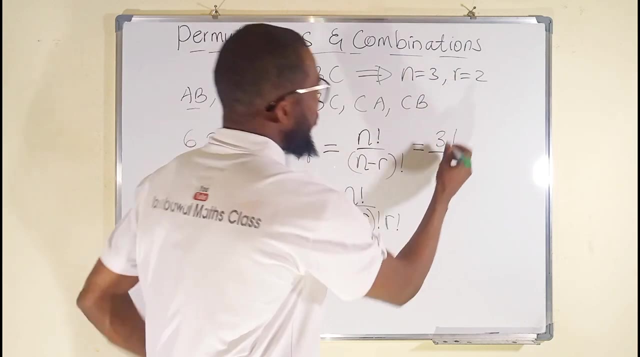 we are going to substitute from this formula to see whether we are going to get 6 and 3 respectively for permutation. this is equal to remember: n is 3, so we have 3 factorial divided by n minus r, R, r is 2,. 3 minus 2, okay, let me even write it: 3 minus 2, also factorial. this is equal to: 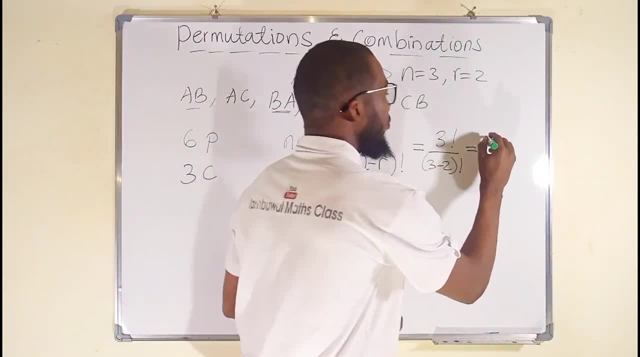 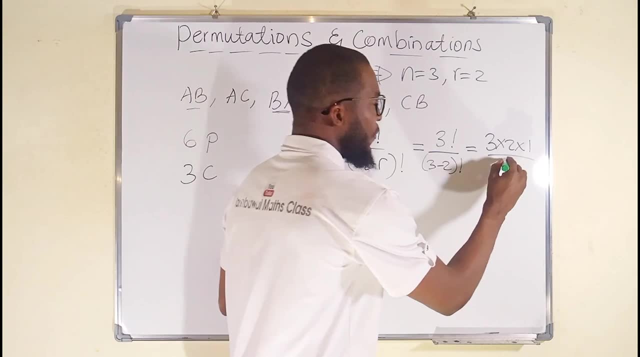 3 factorial means 3 times 2 times 1, so we have 3 times 2 times 1 here. divide by 3 minus 2 is 1, so we have 1 factorial. remember 1 factorial and 0 factorial are all equal to 1,. 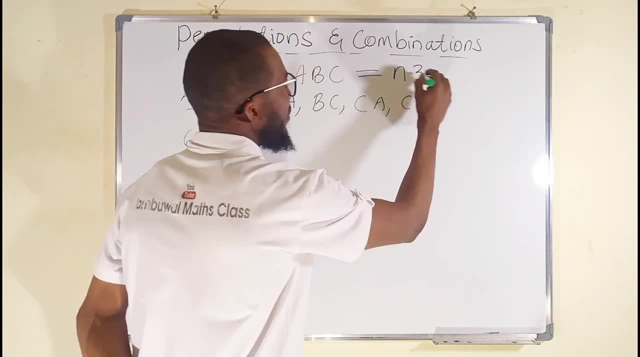 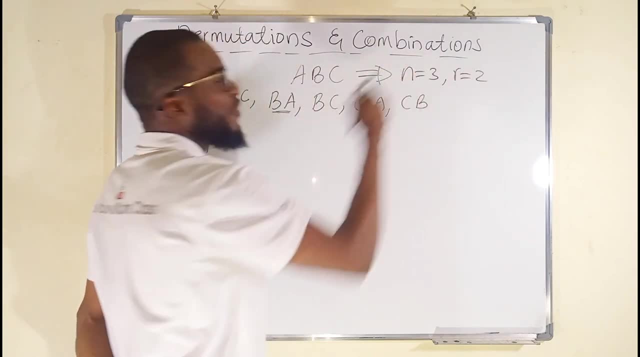 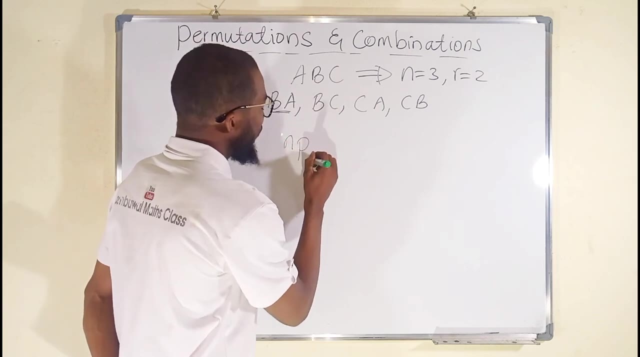 where N here is equal to three And R N equal to three And R equal to two, because we are choosing two out of three. So for permutation we have N permutation R, which is equal to N factorial. Remember we know what N factorial is all about. 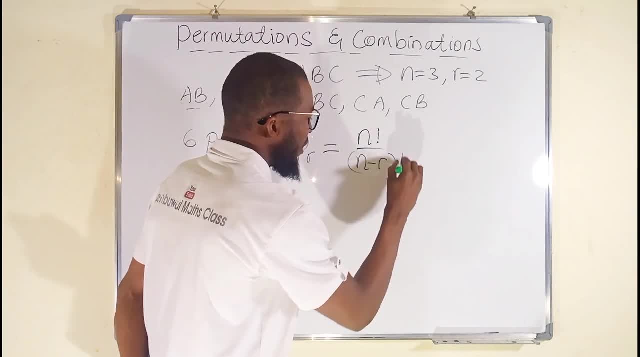 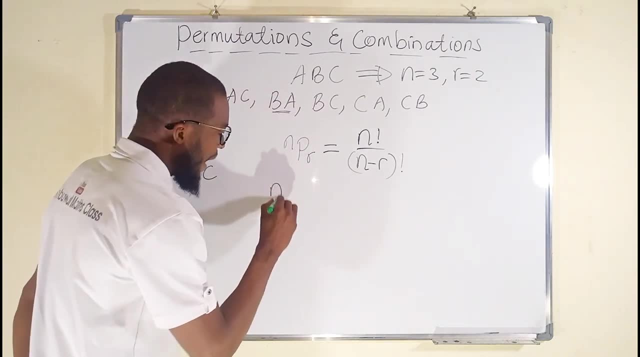 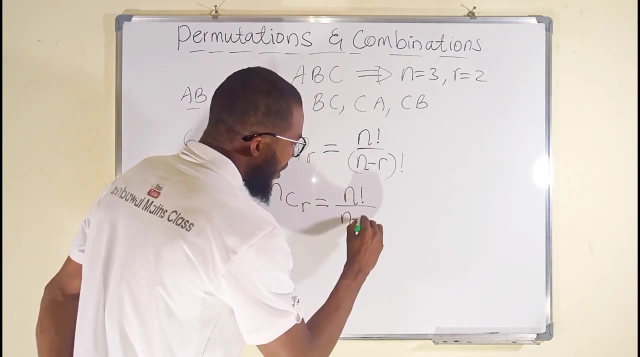 Divide by N minus R factorial. This is what defines permutation. This is what defines permutation. This is what defines permutation. But for combination we have N. choose R is equal to N factorial. divide by N minus R factorial. Then also multiply by R factorial. 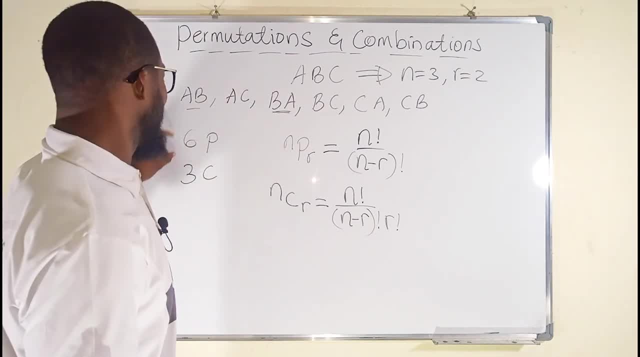 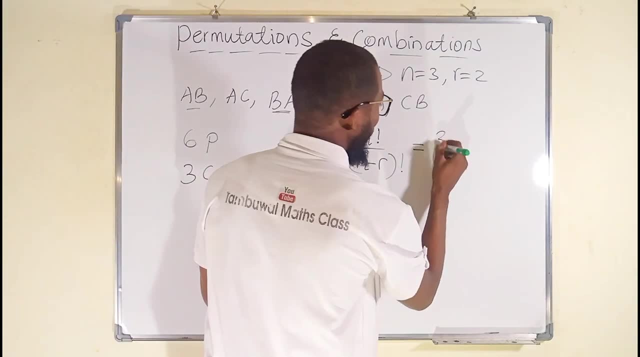 We are going to substitute from this formula to see whether we are going to get six and three respectively For permutation. this is equal to remember: N is three, So we have three. factorial divide by N minus R, R is three. 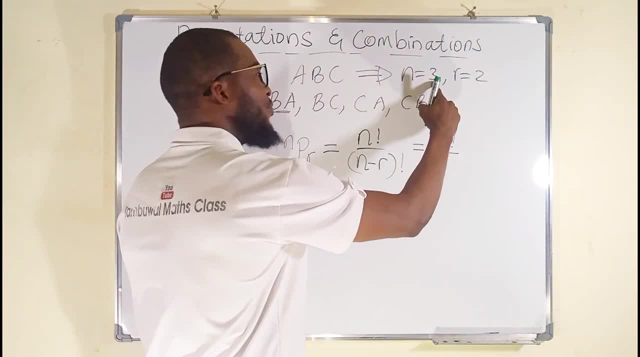 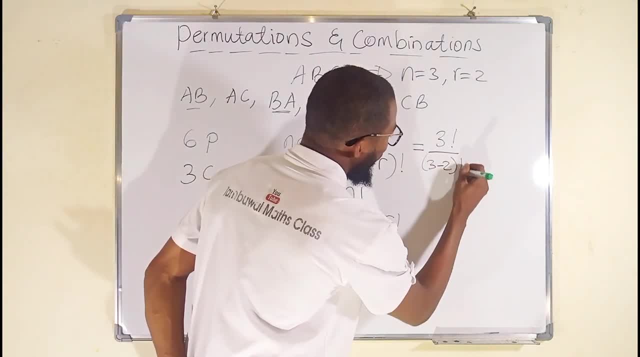 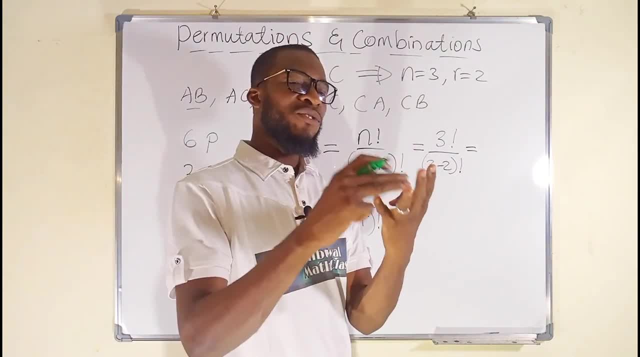 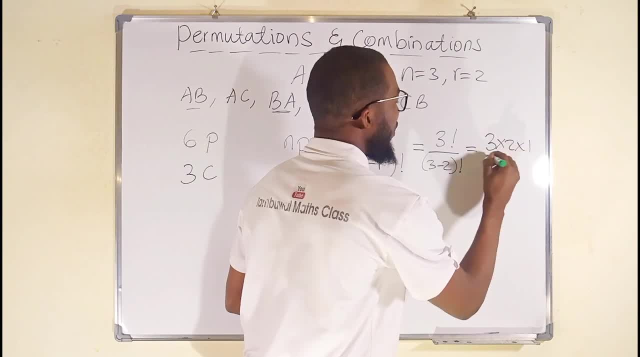 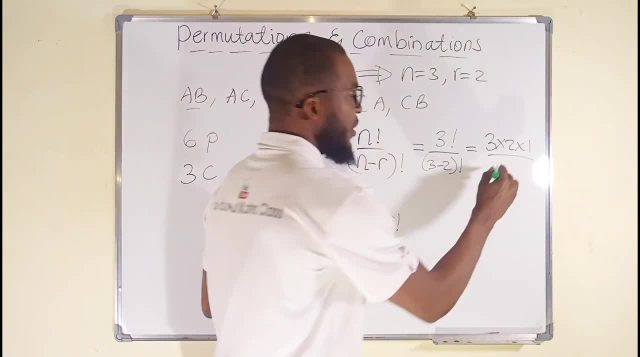 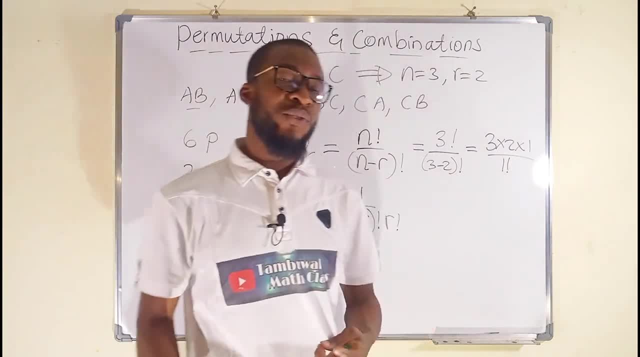 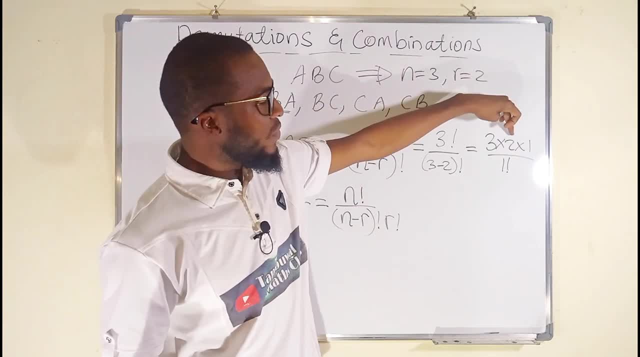 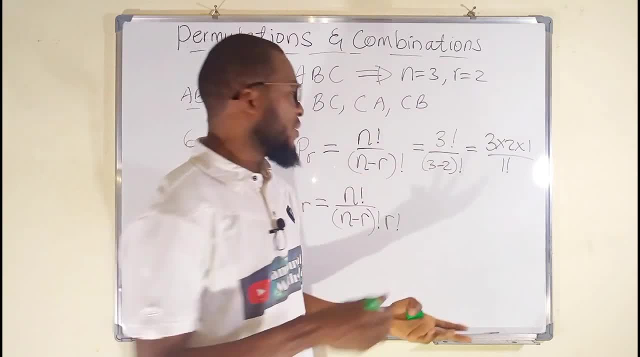 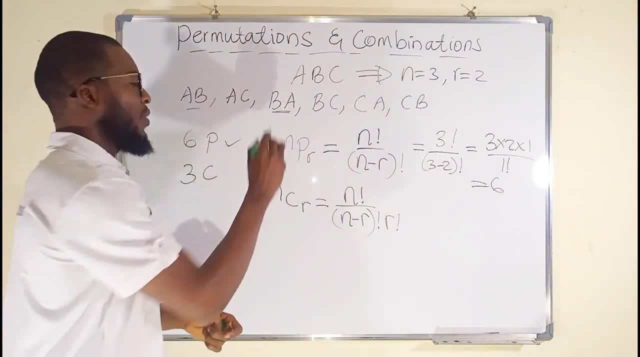